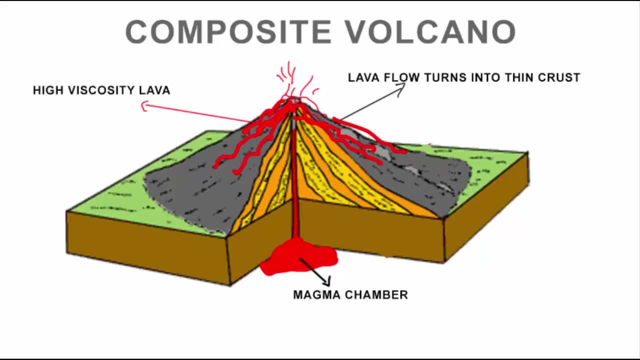 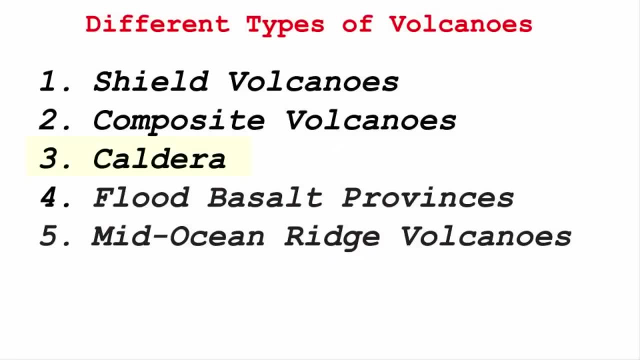 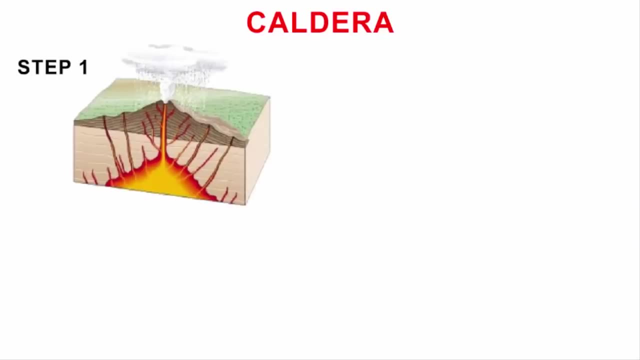 These volcanoes often result in explosive eruptions. Along with lava, large quantities of pyroclastic material and ashes find their way to the ground. The third one is the caldera. These are the most explosive volcanoes. They are usually so explosive that, when they erupt, they tend to collapse on themselves. 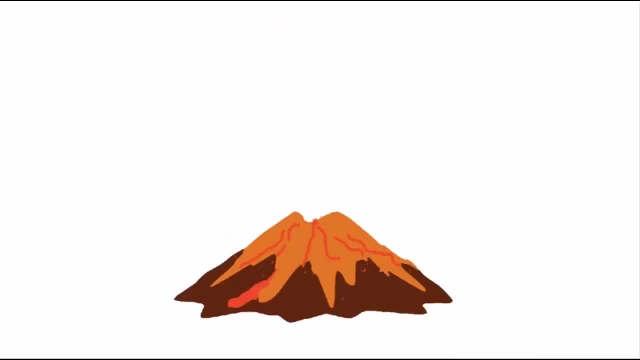 rather than building any tall structure. When we say explosive, we mean how hard it shoots upwards, Because if the eruption is not explosive, Then the lava will erupt And the lava will flow in a nice river format. Explosive eruption means shooting harder upwards. 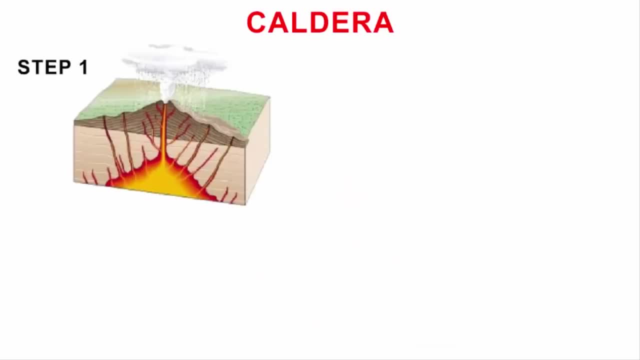 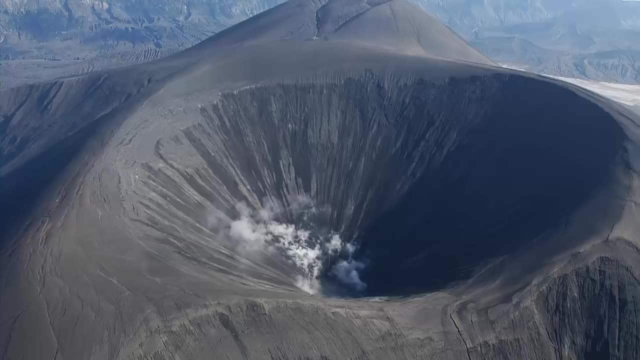 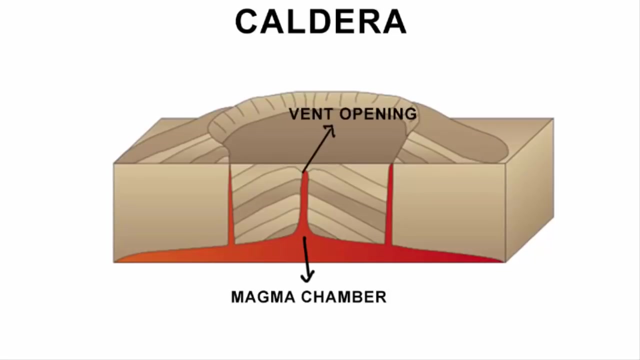 Remember that. So caldera are explosive and because of that, the vent opening collapses on itself. That creates a depression, and this depression is called calderas. Their explosiveness indicates that the magma chamber supplying the lava is not only huge, but is also in close vicinity. 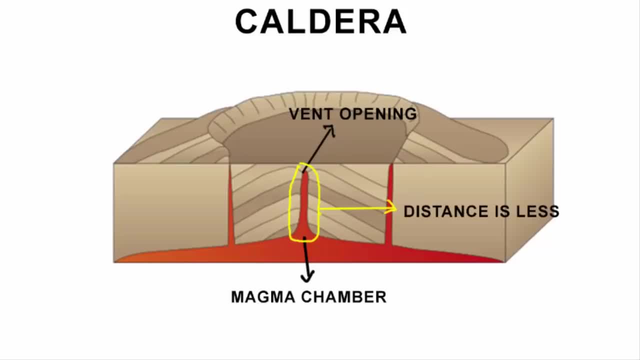 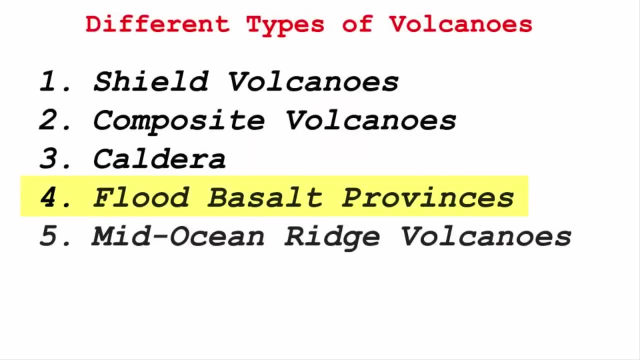 Because the gravity will not allow the lava to go very high. Therefore, The distance between the magma chamber and the vent opening of the volcano has to be close. The fourth one is the flood basalt provinces. If you look at the words flood, basalt and provinces, they speak about riverbed sort. 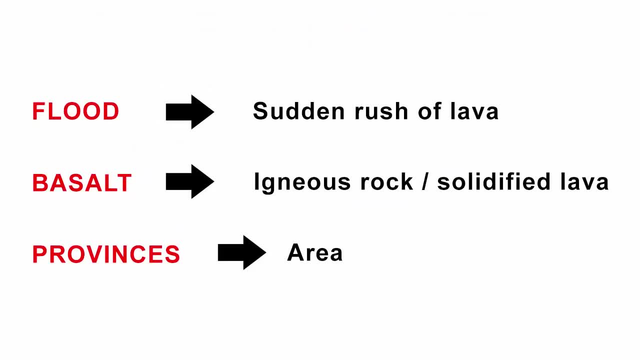 of physical appearance. Let me just break it down for you. By the word flood we mean a sudden rush of something. in this case it has to be lava. Then basalt is a dark-coloured, fine-grained, igneous rock which is solidified state of. 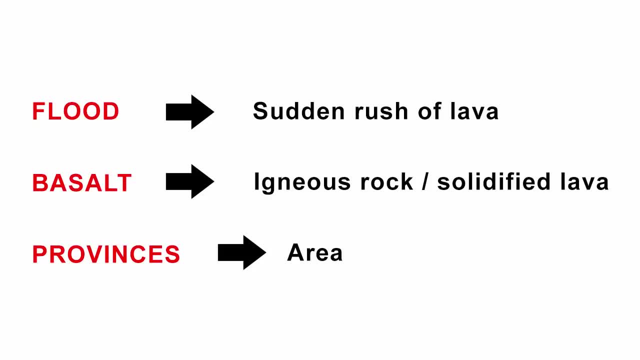 lava And province is called an area. Then basalt is a dark-coloured, fine-grained igneous rock which is solidified state of lava And province is called an area. Then basalt is a dark-coloured, fine-grained igneous rock which is solidified state of lava. 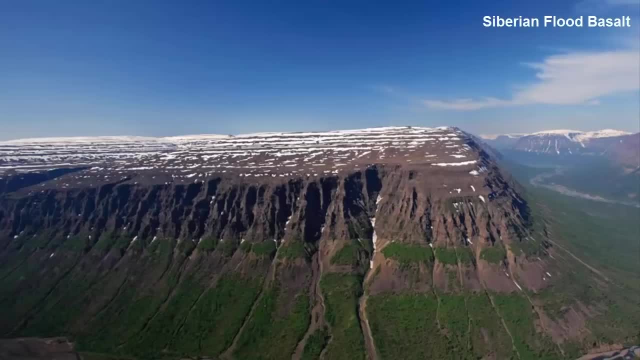 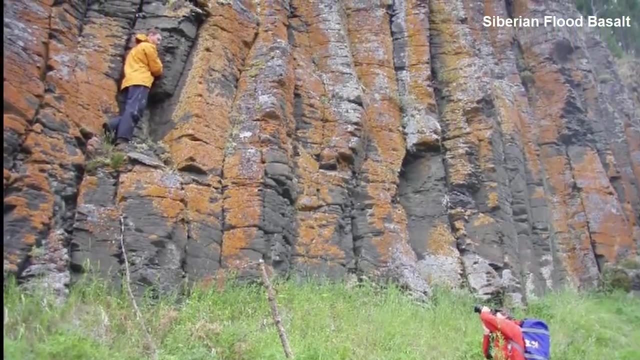 Then basalt is a dark-coloured, fine-grained igneous rock which is solidified state of lava. So collectively, the term flood, basalt provinces means outpour of highly fluid lava that flows for long distances, maybe some thousands of square kilometer, forming a terrain, a landscape. 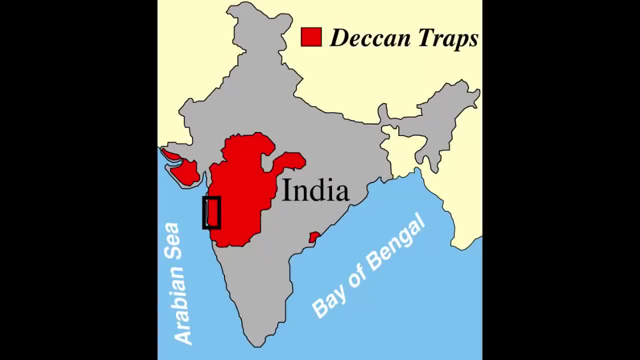 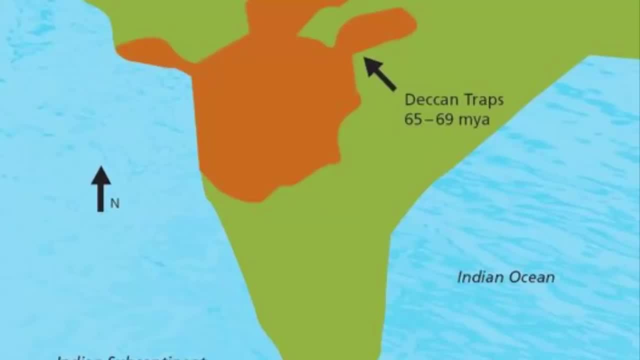 The Deccan Traps from India, presently covering most of the Maharashtra Plateau, are a much larger flood basalt province. That's why this region is made up of vast sheets of massive granite rock, gneiss, quartzite, etc. 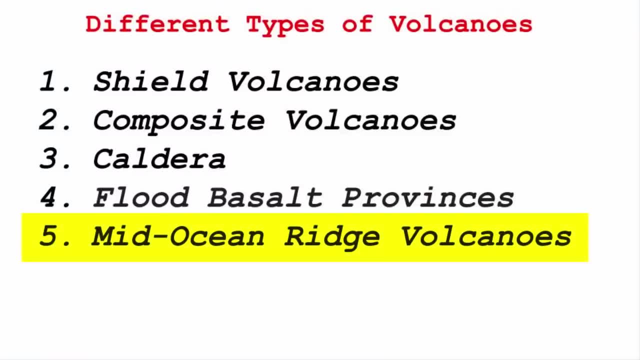 The fifth and the last one is the mid-ocean ridge volcanoes. The fifth and the last one is the mid-ocean ridge volcanoes. A mid-ocean ridge volcano is a large deep-water volcano. A mid-ocean ridge is an underwater mountain range formed by plate tectonics.